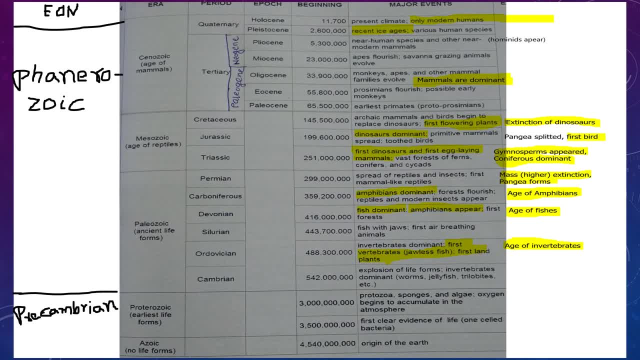 oxygen begins to accumulate in the atmosphere, atmosphere. so you should remember here first clear evidence of life and accumulation of oxygen in pre-cambrian. okay, but this is not that much of important. mostly questions are asking from phanerozoic eon. so let's see. 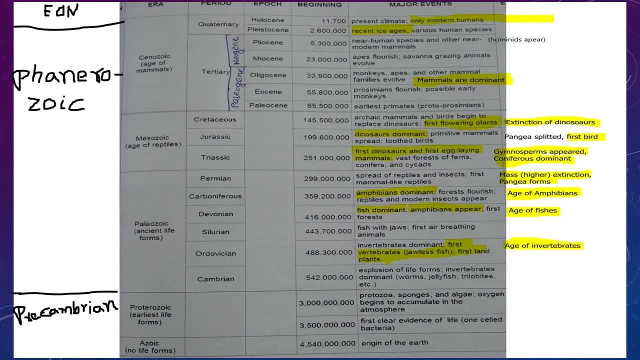 what are the events of phanerozoic eon? in phanerozoic eon there are three events of the eons. they are the eras paleozoic, mesozoic and xenozoic. reason is xenozoic, oldest is paleozoic. in paleozoic era, six periods are there. 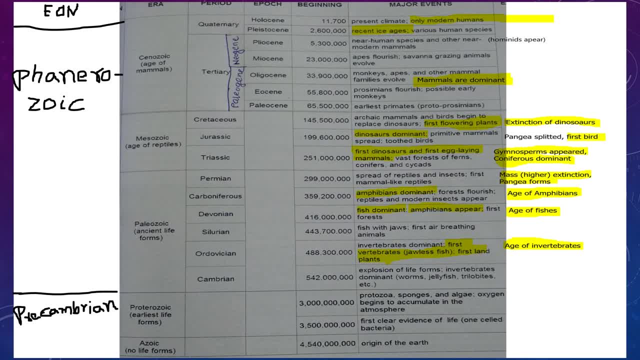 cambrian, odovician, sidurian, devodian, carboniferous and pormian. let's see what are the events of earth. cambrian period. what are the events of earth cambrian period? explosion of life forms, invertebrates, dominant Invertebrates like worms, jellyfish, trilobites. 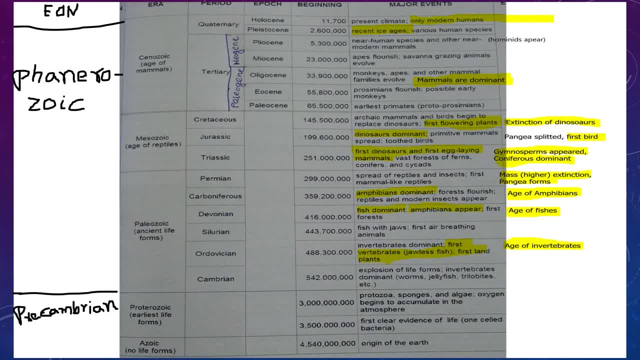 are dominant. So here you have to remember: explosion of life forms occurred at cambrian period. Okay, next is autopsian period. In autopsian period invertebrates dominant. So we can say it is the period of age of invertebrates. So age of invertebrates is: 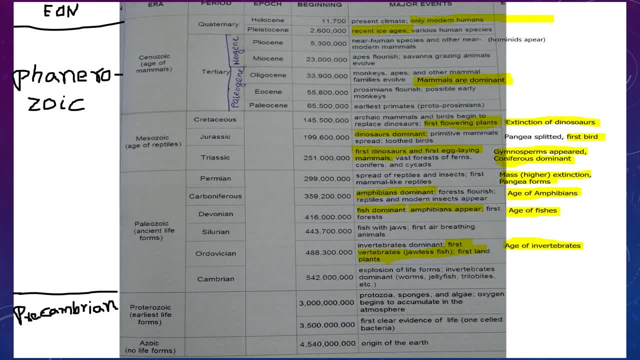 odovician. Next, first vertebrates, jollus fish, appear In odovician. first land plants appear. So here you have to remember: first vertebrates, age of invertebrates, first land plants in odovician. 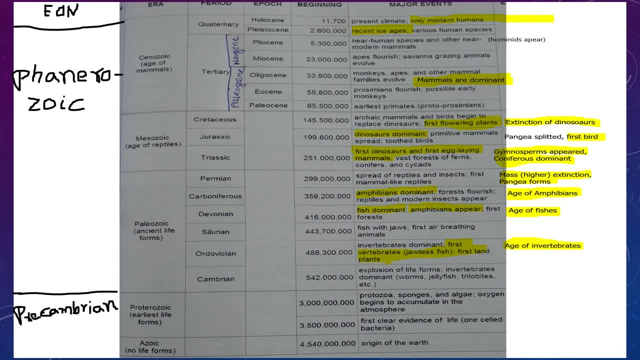 Here I am highlighting with yellow color is most important. At least you should remember that points. If you can remember all the events means that is very good, but at least you should remember this highlighted events. So here in odovician you have to remember age of invertebrates: first land plants. 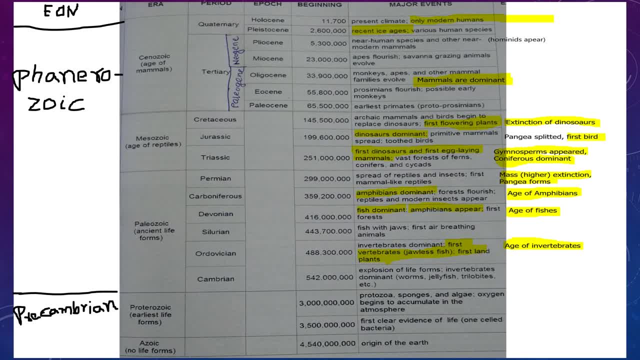 and first vertebrates. Next is silurian- In silurian fish with jaws first breathing animals. Next is devonian fish dominant. So we can say it is age of fishes. So age of fishes is devonian, Ambivians appear First. ambivians appear in devonian First. 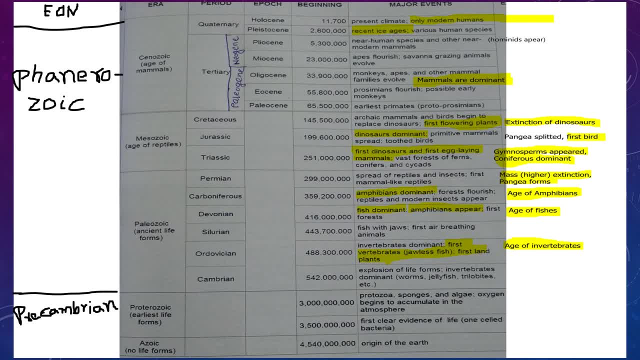 forest. Okay, next is carboniferous Ambivians dominant. So we can say it is age of ambivians Forests, flourish Reptiles and modern insects appear. Next is permian In permian period, spread of reptiles and insects. First, 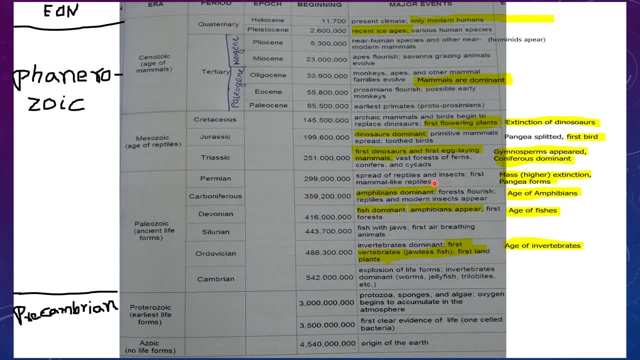 animal like reptiles. Mass or higher extinction: Pansia forms Here. mass or higher extinction is very, very important. One question asked. I do not know which year it is asked, but this is very, very important. I think it was in June 2008.. There was a question Highest. 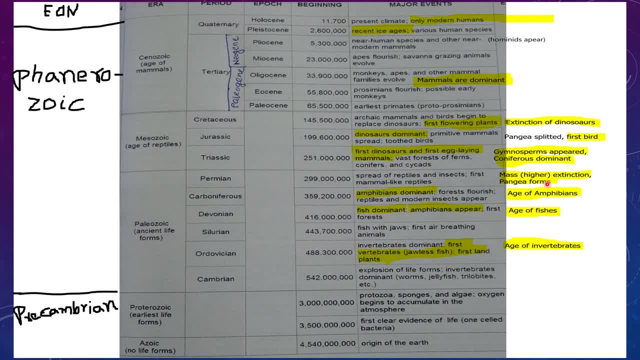 extinction during the history of earth was observed during like that, That is permian. So you should remember that. Next is Mesozoic era. In Mesozoic era, three period are there: Triassic, Jurassic and Cretaceous. 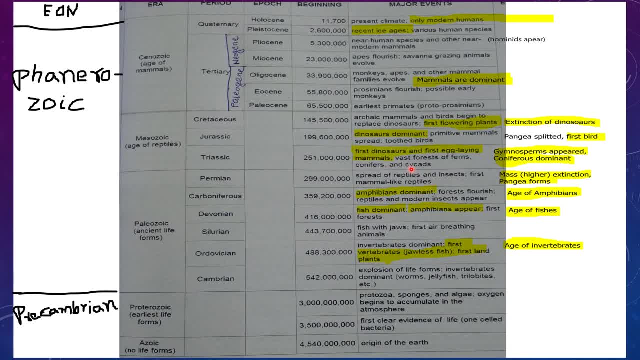 First dinosaur and first egg-laying mammals. Wast forest of ferns, conifers and cicad. Gymnosperms appear, Coniferous, dominant Here, you have to remember. first dinosaur appeared in triassic. Gymnosperms appeared at triassic. Coniferous are dominant in triassic. Okay, 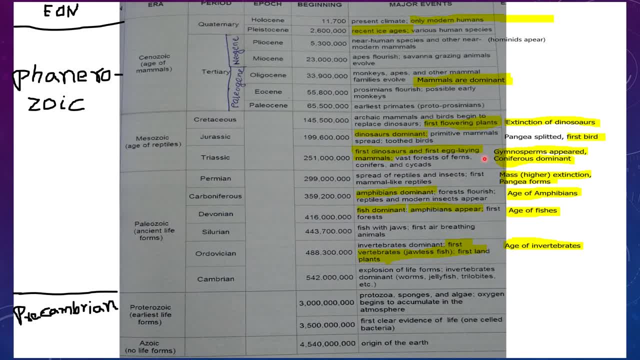 Okay, next is Jurassic. In Jurassic, dinosaurs are dominant. This is the golden age of dinosaurs. Don't forget that. You can relate it to that Jurassic Park movie that is related to a dinosaur, So you can remember this like that: First dinosaur, first egg-laying mammals. 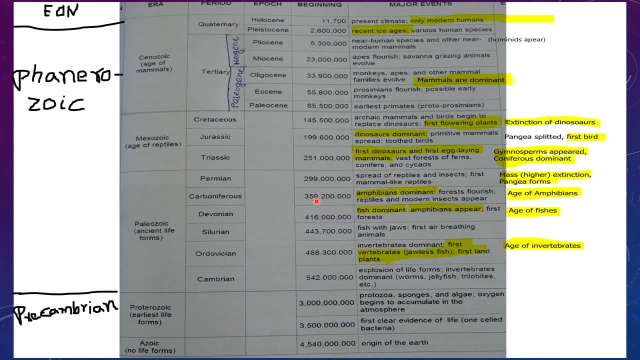 Sorry, in Jurassic dinosaurs are dominant Primitive mammals, spread Tooth birds, panchea splitter, first bird. So here you have to remember golden age of dinosaurs and first bird in Jurassic. Next is Cretaceous. In Cretaceous archic mammals and 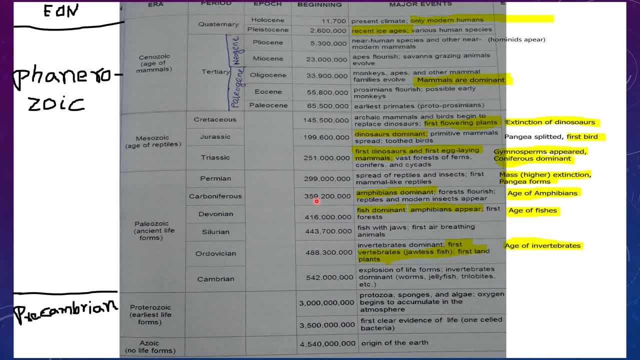 and birds begin to replace dinosaurs. First, flower implants, extinction of dinosaurs. Here you have to remember, first flower implants, that is angiosperms, appear and extinction of dinosaur in Cretaceous. Next is Paleogene Period. In Paleogene Period, in Cenozoic era, there are 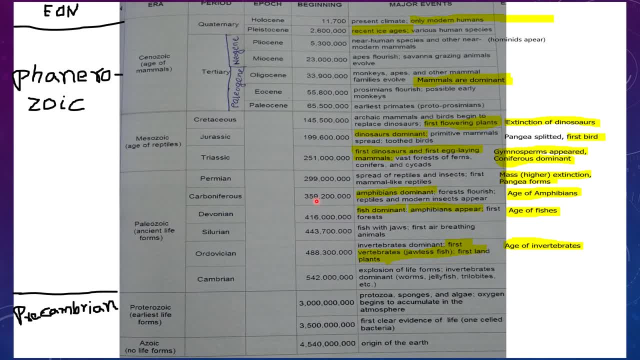 period: Paleogene, Neogene and Quaternary. Paleogene and Neogene, both together we can say tertiary period. In Paleogene period there are three epoch: Paleogene, Eogene and Oligogene. Let's see what are the events of Paleogene Earliest primate. or we can say: proto-prosimians appear In Eocene. prosimians flourish, possible early monkeys. In Oligocene, monkeys, apes and other mammals- sorry, other mammals' families evolve. So in Oligocene mammals are dominant. Here you have to remember. 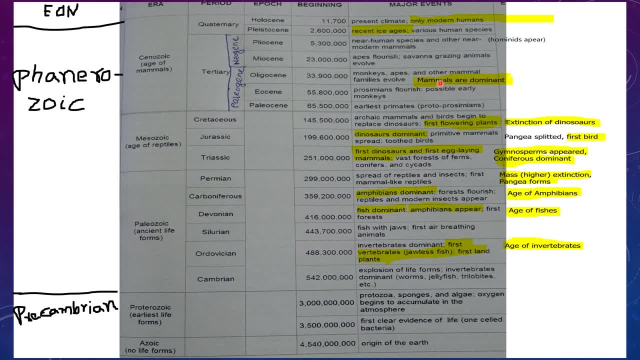 mammals are dominant in Oligocene, Next is Neogene. In Neogene Period, two epoch are there: Neogene and Paleogene. In Neogene apes flourish savannac-greasing animals evolve. In Paleogene near humans, species called hominidians and other near modern mammals appearäm. 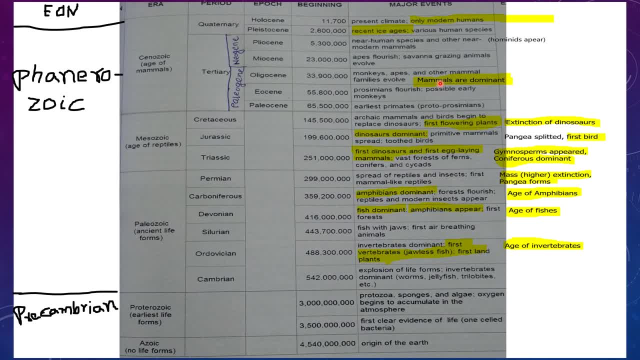 Next is Quaternary Period. In Quaternary Period, two epochs are there: Pleistocene and Holocene. In Pleistocene, recent ice ages, various human species evolved. Next is Holocene, Epoch. This is the present climate, only modern humans. So you have to remember these major events in geological time scale. 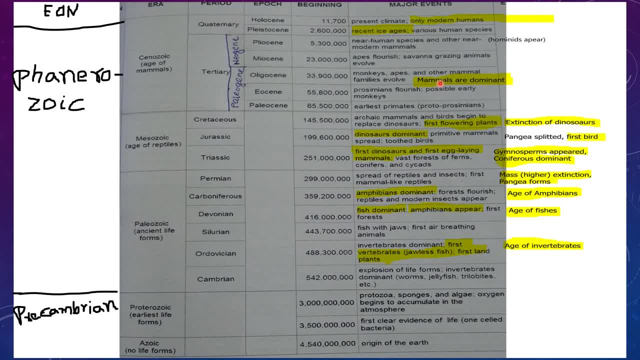 If you can remember all the events means that is very good. If you are not able to remember all the events means you can at least remember some of the important events. Let's see what are the most important events. Let's see what are the most important events. 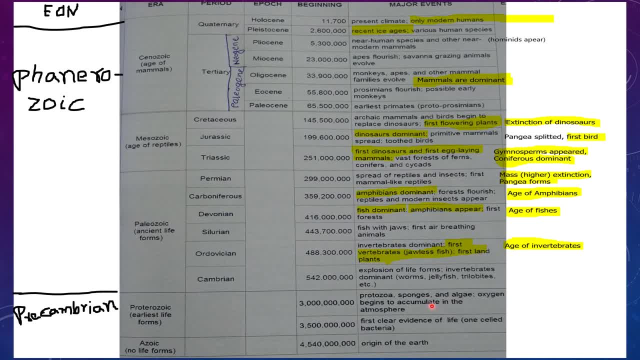 Let's see what are the most important events. One is in Pre-Cambrian, you should remember, first clear evidence of life, That is, Unicellular Bacteria and accumulation of atmospheric oxygen. And in Cambrian, you should remember, explosion of life forms, In Ordovician age, of invertebrates and first land plants. 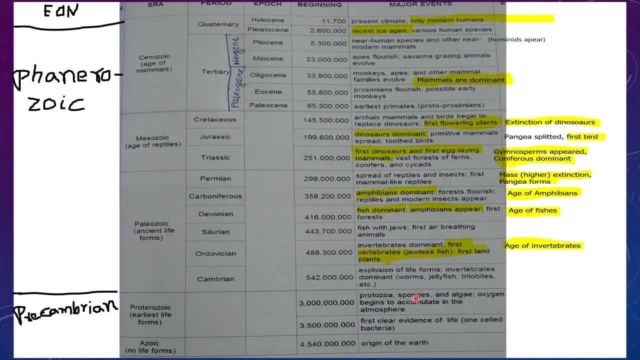 And in Cambrian, you should remember, explosion of life forms. You should remember that In Silurian fish with jaws first, everything, animals Next in Devonian age of fishes and amphibians appear In Carboniferous amphibians are dominant, So it is called age of amphibians. 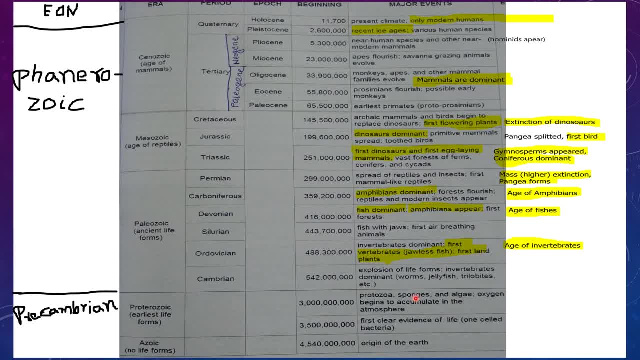 And Forest flourish That is not a forest flourish, That is not that much of improtant. But you should remember at least age of amphibians for Carboniferous Permians mass or higher extinction And or panacea forms. In Triassic first dinosaur appear And the genus forms evolved. 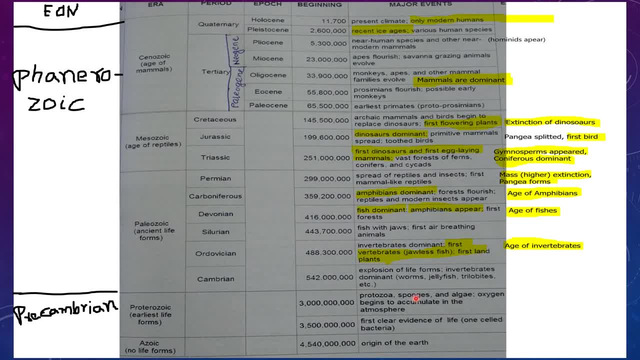 Conifers are dominant In Jurassic, dinosaurs are dominant. First bird evolve And the Pangea split In Cretaceous angiosperms evolve. That means first flowering plants evolve And the extinction of dinosaur. That is very important. Gymnosperms evolved in Triassic and Angiosperms. 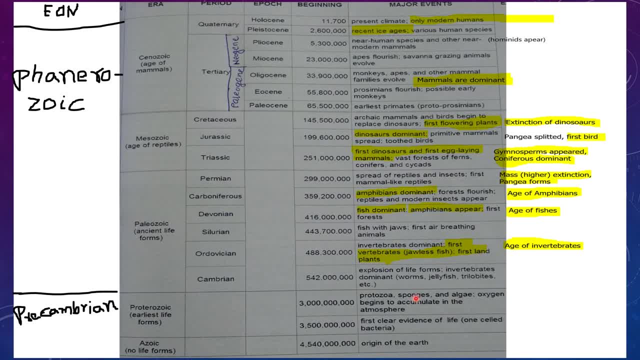 and angiosperms evolved in Cretaceous. don't forget that. next important is: mammals are dominant in Oligocene and hominids in Pleocene. ice age is Pleistocene and modern humans in Holocene. age of reptiles is called Mesozoic era and age. 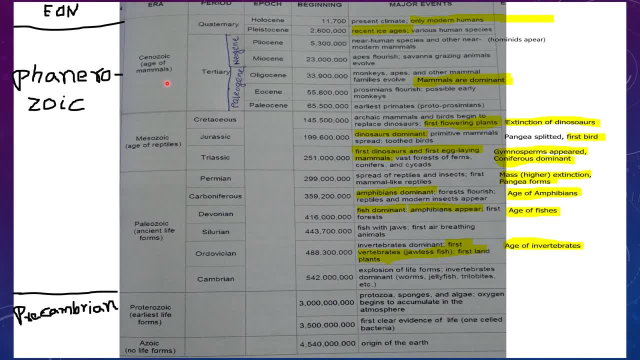 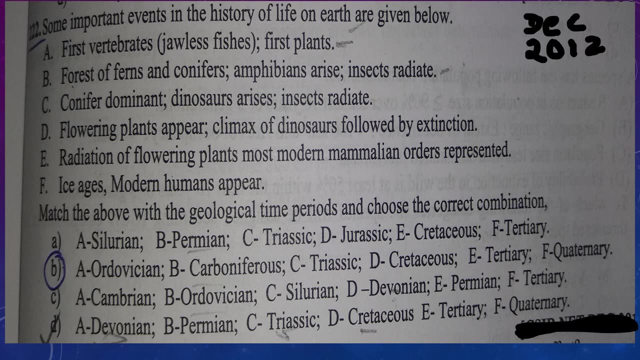 of mammals is Cenozoic. you should remember that also. so let's see one question. this is a question from December 2012. question is: some important events in the history of life on earth are given below statement a- first vertebrates- jawless fishes- first plants. b- forests of 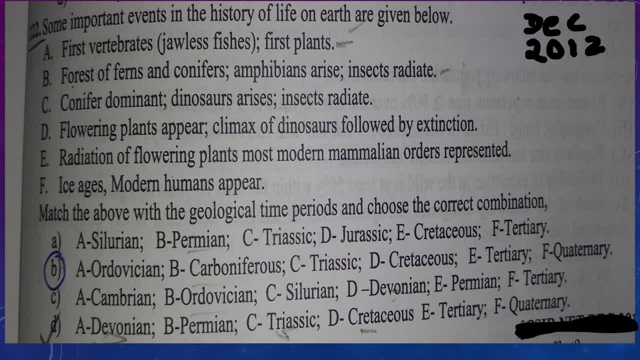 ferns and conifers. amphibians erase insects. radiate 3. corn fern- dominant dinosaur erases insects. radiate d. flowery plants appear climates of dinosaurs, followed by extinction. e. radiation of flowery plants. most modern mammal orders hope that. combination type questions. if combination type questions, there is no need to know everything. you can answer if you know some 10 questions. 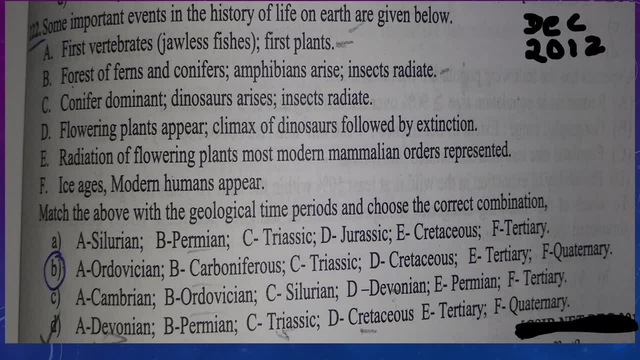 so if you know some questions, dont worry, you can write if you can reach somewhere before workplace statements. If you know some events means you can answer this combination type question. So let's see how to answer this question. The first statement is First vertebrates. 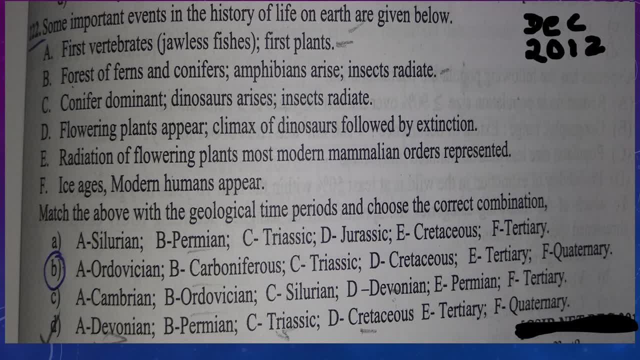 jawless fishes. first plants: First plants appear in odovician. That is the age of invertebrates. At that period only first vertebrates appear. So we can say: this is odovician, So let's see the option. 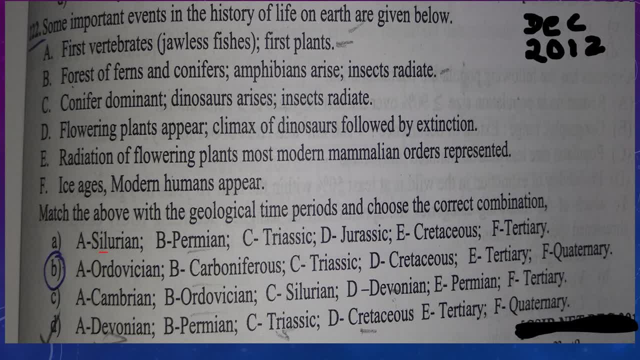 In option A, Silurian. In option B, odovician. In option C, Cambrian. In option B, Devonian. So in option B, odovician, is there Okay? Next B: Forest of ferns and conifers, amphibians arrays. 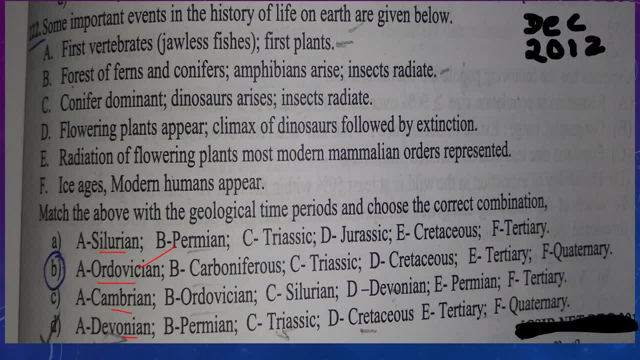 insects, radiates, Amphibians, arrays- In Devonian, But sometimes it is confused with carbon. for us Here there is no Devonian in any of any of these options. First, in option A, Permian. Option B, Carboniferous. 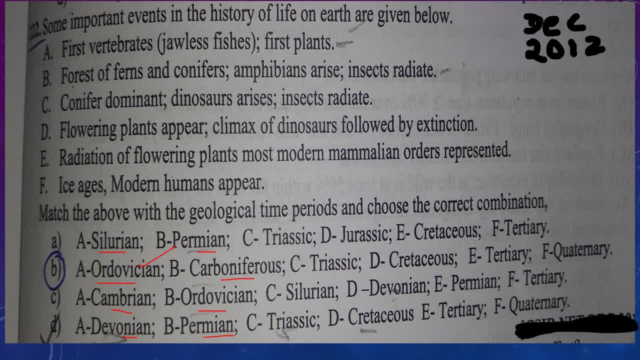 Option C: odovician. Option B: Permian. So there is no Devonian in any option. So there is a confusion. But Carboniferous is there in option B, So let's leave that statement Next go for the. 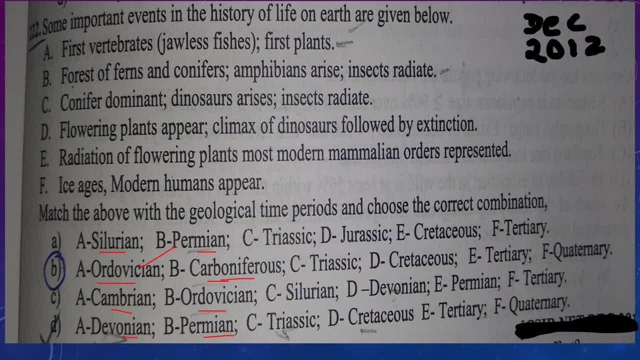 statement C: Coniferous dominant Dionysis arrays- Insect radius Coniferous dominant Dionysis arrays. We can blindly say that it is in triacyc Dionysis arrays in triacic dinosaurs dominant in jurassic extinction of dinosaurs in cretaceous. so we can say that. 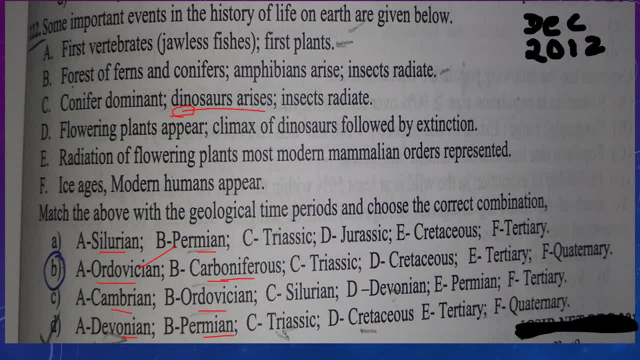 dinosaurs, arrays, conifer, dominant in triassic. let's see the option in option a: c is triassic, option b is c is triassic, option c is silurian, option d is also triassic. so here in three options, triassic is there, okay. next d: flowering plants appear. climax of dinosaur, yes, followed by extinction. 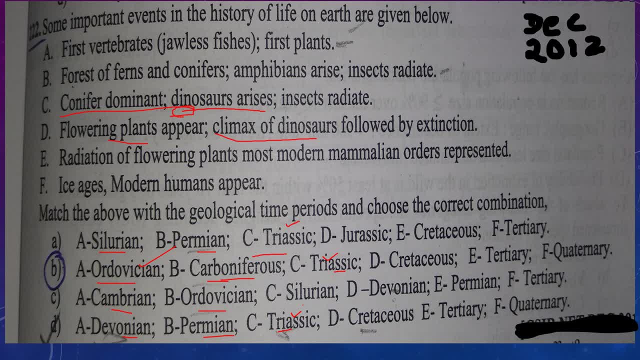 extinction of dinosaurs and angiosperm, that is, flowering plants, appear in cretaceous. let's see the options in option a, d is jurassic, so this is not correct. jurassic dinosaurs are dominant, so jurassic is not correct. so option d is cretaceous, is there? 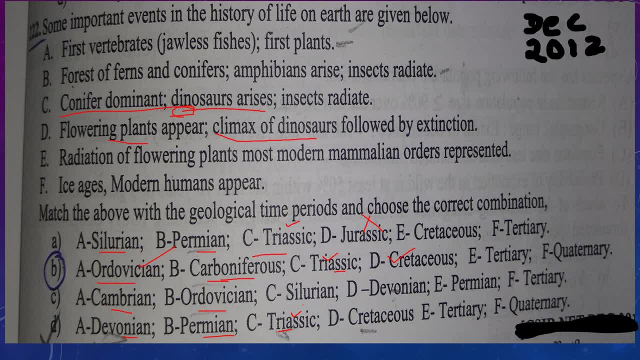 this is correct. you know this is divine or devonia, so this is also not correct. in option d, it is there. so in option b and option d, cretaceous is there. next, go for statement e: radiation of flowering plants- most modern mammals. order represented: ejo marmal堡. 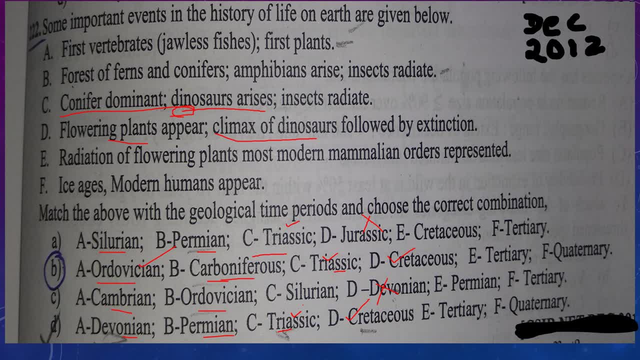 now the mass cation bill. you see it is way high framerato. maher àylabos of mammal is tertiary period, or we can say it is in oligosine epoch or paleogene period. so here this given tertiary age of mammals is tertiary here. 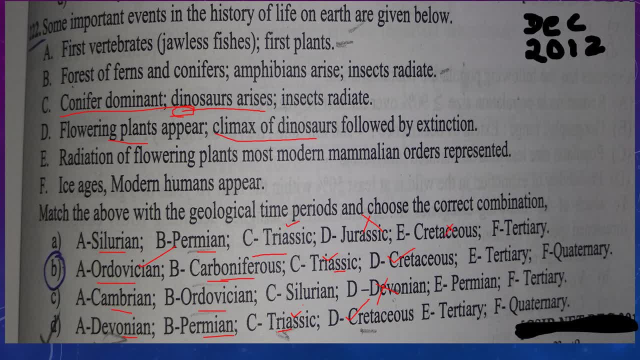 it is Cretaceous, it is tertiary, it is a Permian, it is tertiary if it. if you are not sure means. if you are not sure means, let's leave that statement and go for the next statement. option F is ice ages or modern human. appear modern humans in? 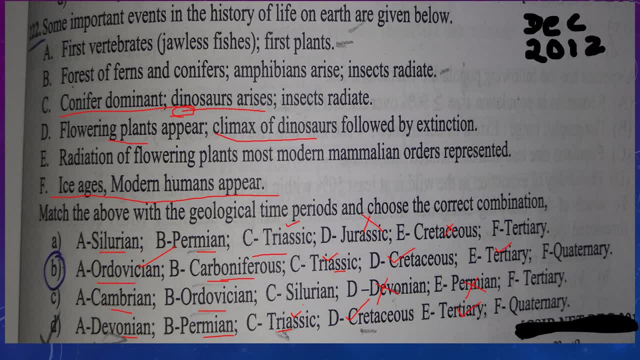 quaternary: the recent period. so let's see. option A: tertiary is the, so it is not correct. quaternary is in option B, that is correct. option C: tertiary- not correct. quaternary is the in option D, that is correct. so let's see here we are confused with this carboniferous. 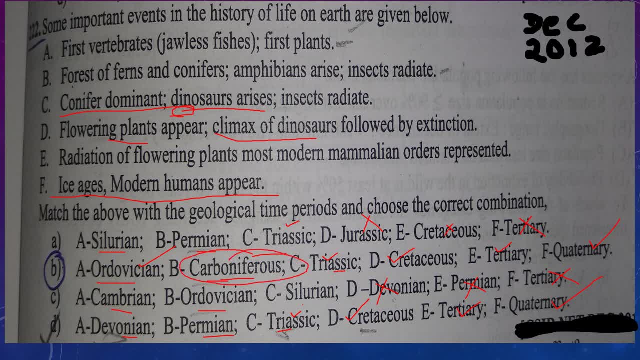 and to be were not away from. this is not correct. no, first, France is not in Devonian be snow, so not correct. a means 또 ню carboniferous. So the answer is option B: A Odovician, B- Carboniferous, C- Triassic. 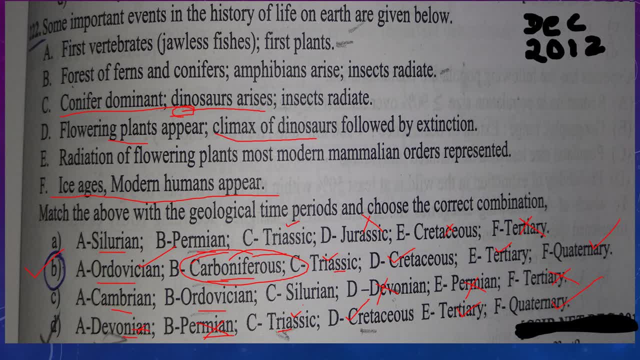 D, Cretaceous E. Tertiary F, Cardinary. Let's see another method to answer this combination type question. Before that, I want to erase this one. Let's erase this one. Okay, let's see. First statement: is first vertebrae joules fissures or first vertebrae? 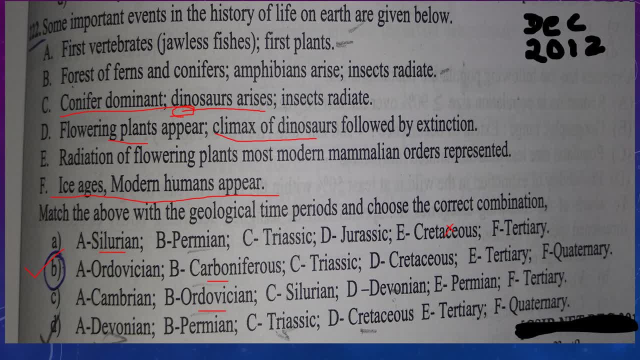 First plants. If you know, that even means you can answer here. slash search, Otherwise you can leave that one. Next, forest of ferns, amphibians, rats. That is also confused, means Leave that statement also. So C statement is dinosaurs, rats, conifer dominant. So we can blindly say that it is. 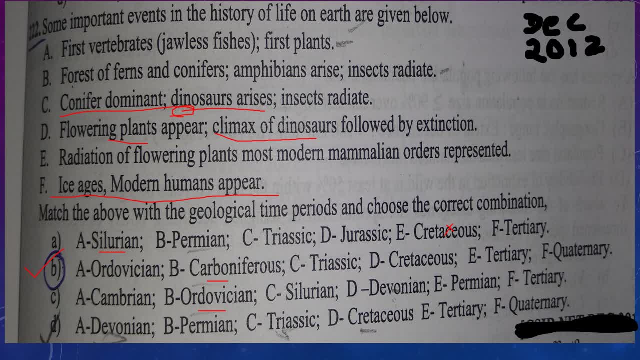 In triassic. So let's see where triassic- Option A is triassic- is there. Option B is there. Option D is also triassic- is there. Next is flower implants appear, Extinction of dinosaur That occur in Cretaceous. So where it is Cretaceous, Here Cretaceous is there. Here, Cretaceous is there. 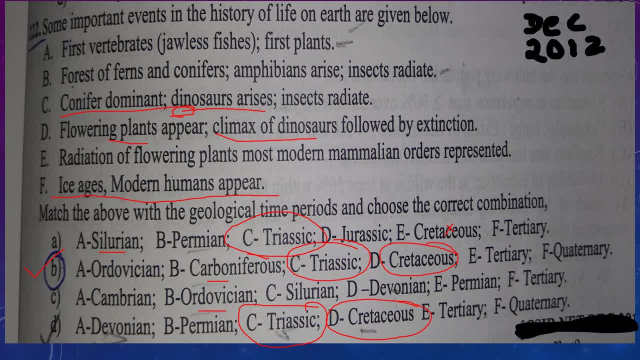 Here, Jurassic is there, So the Option A is incorrect Here. Option C is also incorrect. Okay, Next go for the next statement. Radiation of flower emblem on most modern mammals' odors represent Age of mammal is tertiary. 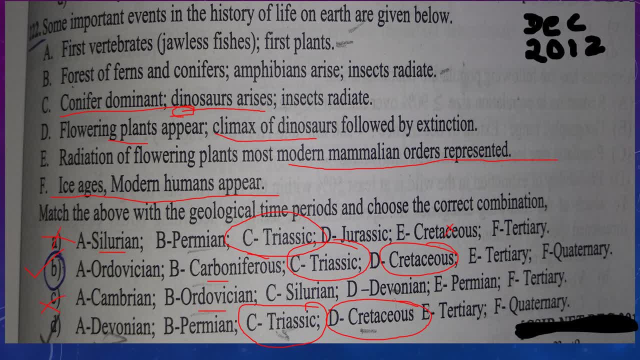 Okay, Mammals are dominant in paleogene. Okay, So we can say tertiary. So let's see where tertiary is there. Already we confirmed that option A and C are incorrect, So let's see option B and D: Here tertiary is there, And here tertiary is there. 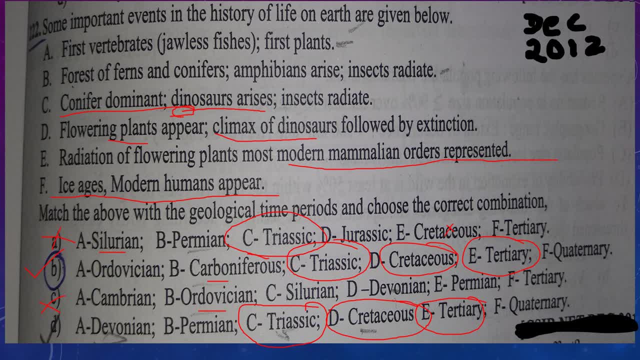 Okay. Next is: next is ice ages, Modern humans appear. Let's see the statement: Modern humans in quaternary. Okay, Ice ages is also there. Okay, Next. go for the next statement. Radiation of flower emblem on most modern mammals' odors represent Age of mammal is tertiary. 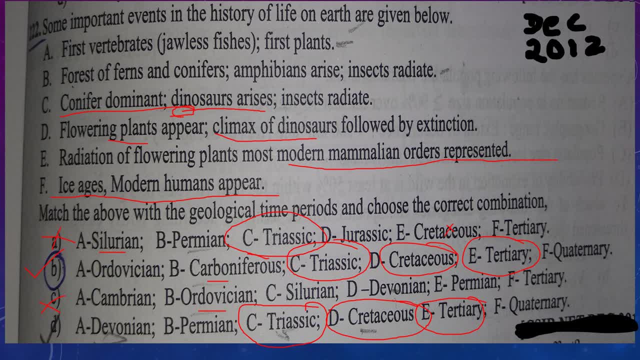 Also in quaternary period. So let's see the options Here, quaternary is there, And here is also quaternary is there. Now we are in confused state because option C, D, E and F are correct in option D. 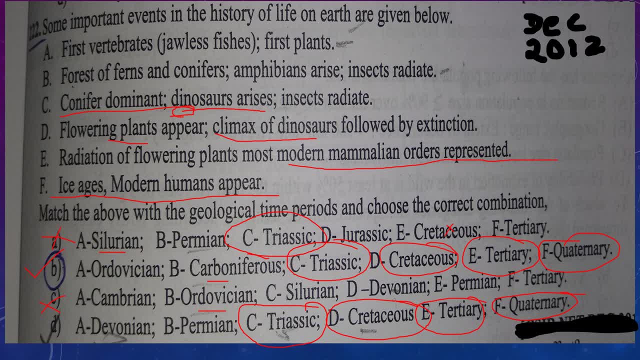 Please make your postion. So let's go for the statement A and B: Fast vertebrates and fast plants. Let's see the option: Odovician is there and Theodon is there. We know that in Devonian That is the age of fishes and fast ambibians. 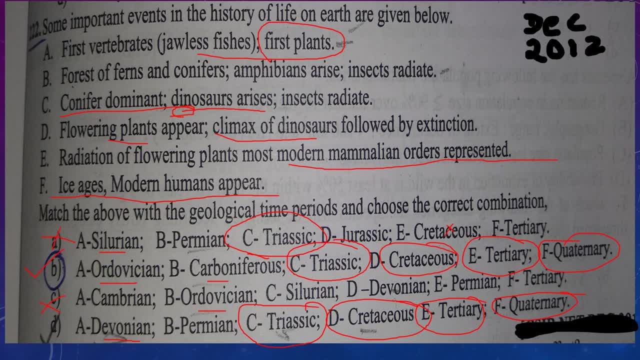 Okay, First ambivalence in Devonion. That is the age of fishes. That means fish is dominant in that period. Okay, So we can confirm that fish evolved First. fish formed in period before that. So we can say that option D is incorrect. A is not Devonion. Okay. 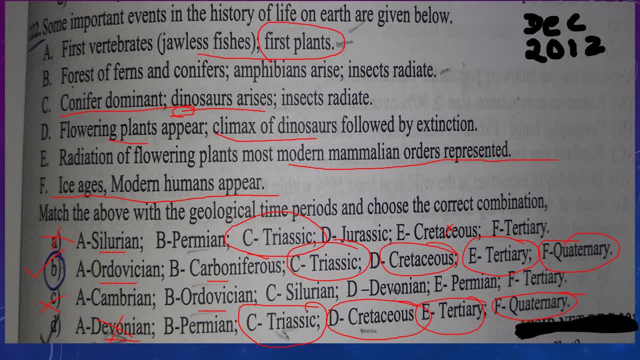 Okay, And So So, So, So we can blindly say that option B is correct. Let's see the option statement B also: Forest ferns, corn ferns. ambivalence arrays in such radius Here we have confused with Carboniferous and Devonion, Because in Devonion we told that ambivalence evolved in Devonion and age of ambivalence That means ambivalence dominant in that period.